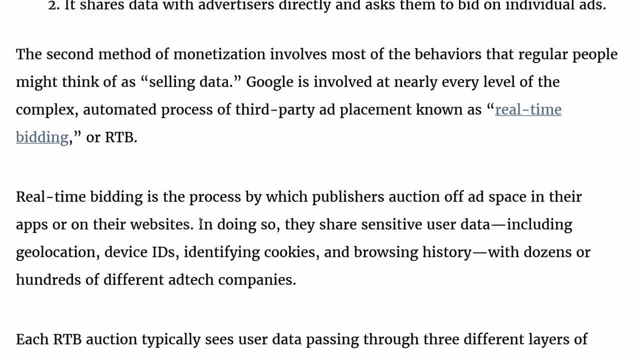 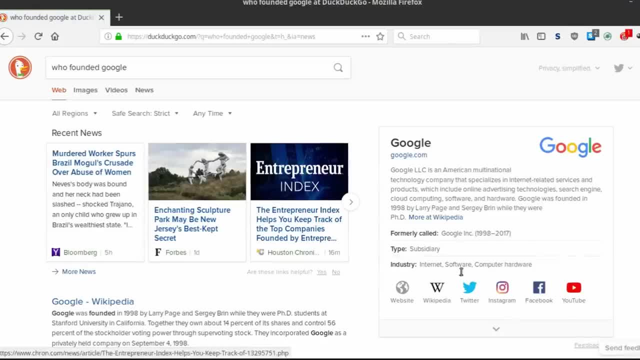 it and then release these profiles to data brokers and advertisers. The easiest way to start protecting your search records is to switch to DuckDuckGo. No service mentioned here is gonna be bulletproof or perfect. DuckDuckGo is no exception. But 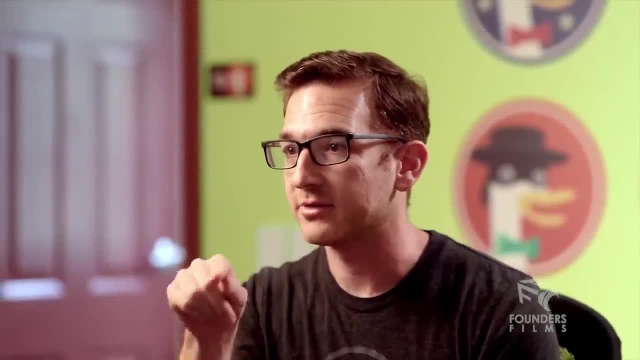 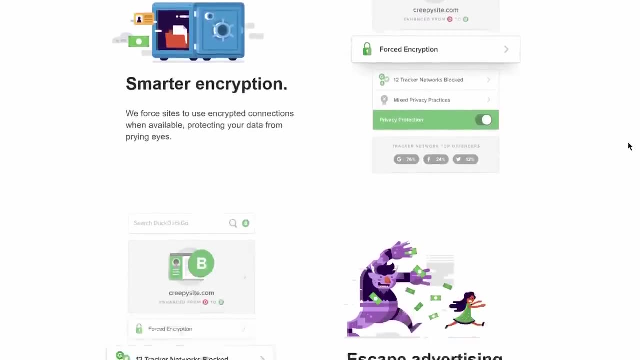 its business model is based on no data collection. There is no profiling or spying on who you are or what you do And, most importantly, DuckDuckGo doesn't log what websites you go to from your search results. DuckDuckGo has a mobile browser available for iPhone. 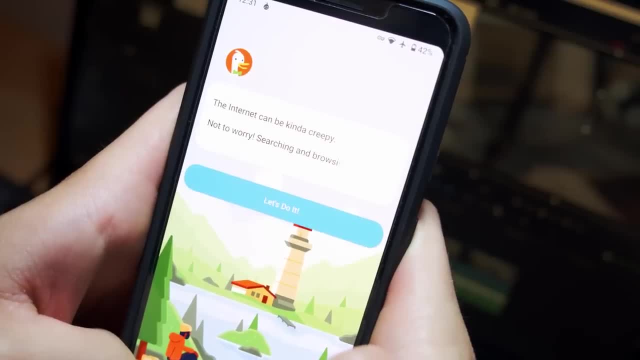 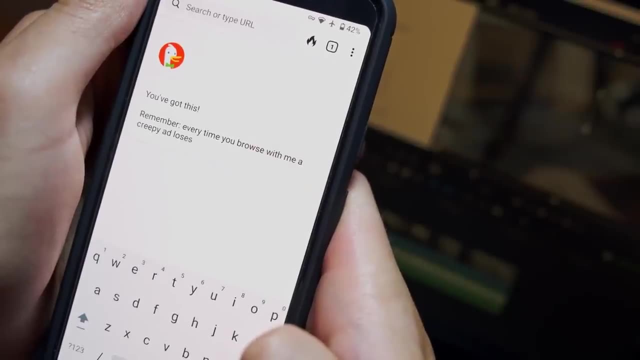 and Android. It's also on FDroid, which means it's fully free and open source. Best feature is that it burns your browser data so that nothing is remembered that websites you visit could later track On all the other browsers you use. change your default search engine to. 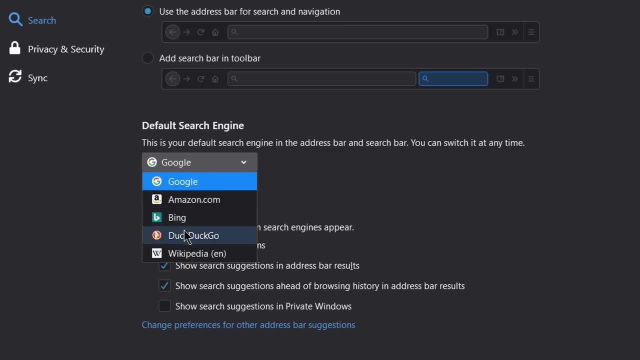 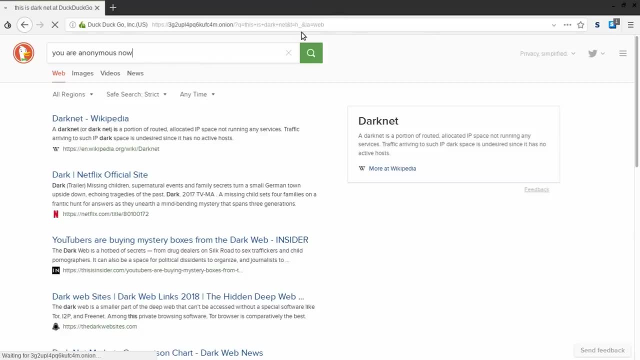 DuckDuckGo and use Google only when you can't dig relevant results on the duck Pro tip. to pull Google results anonymously, use Starpage. Another cool thing about DuckDuckGo is that it has an Onion service, which is a perfect segue to our next section. 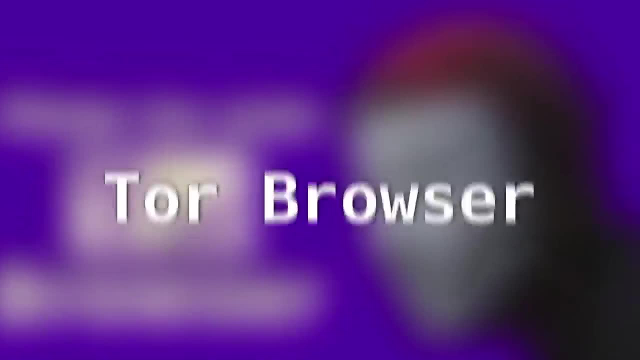 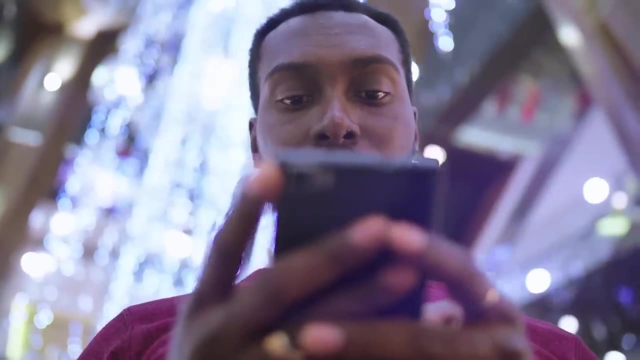 16. Step 2. Tor Browser. The second most valuable privacy asset is your browser history. Everybody is spying on your browsing: Your internet service provider, your browser, the websites you visit and even those you don't visit. The most effective way of securing your browsing records is to. 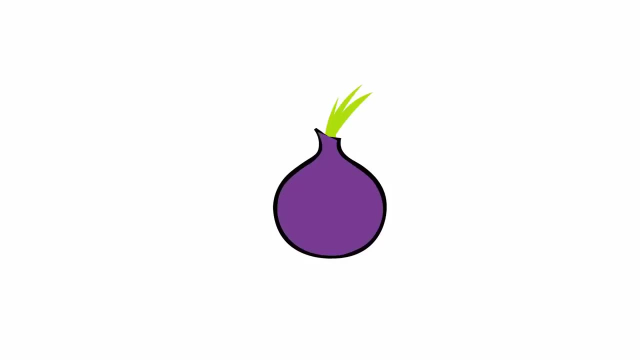 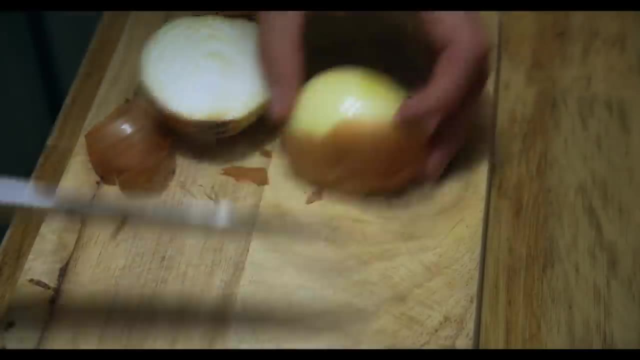 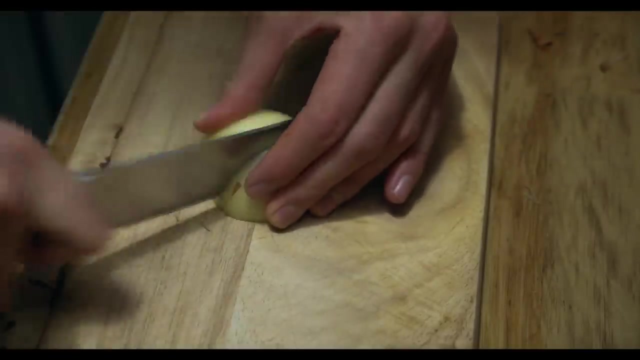 kill all of these threats with one shot, Introducing Tor Browser Available on all main platforms except for iOS, where it comes as Onion Browser. Tor Browser erases your fingerprint, hides your traffic from your IP and changes your IP address in such a way it can be traced back to your true location. 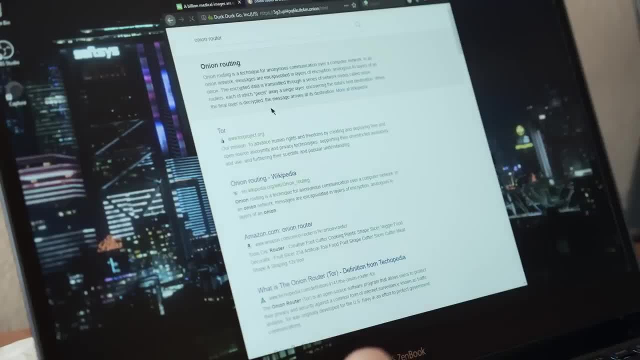 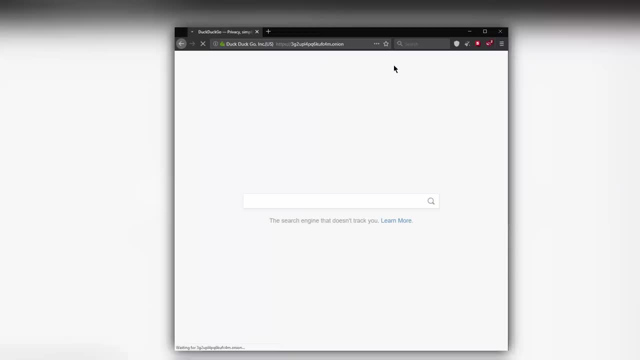 by website you visit. Tor Browser uses DuckDuckGo as a default search engine. stores no browser history, so you have to use bookmarks to remember websites for later and you can have your traffic fully encrypted by visiting Onion websites like DuckDuckGo Onion service, thus taking your 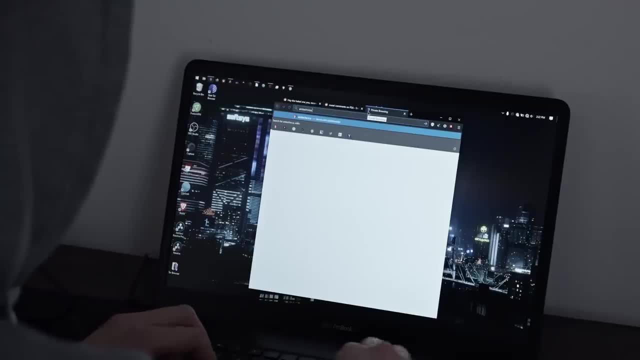 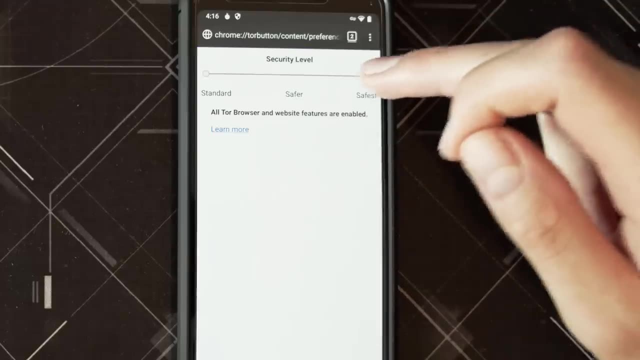 traffic completely off the grid. When using Tor, it's important not to break these essential offsite rules. Do not change any Tor browser settings, Install plugins, install apps and install your own website. The only settings you can change are security settings and requesting Tor bridges. 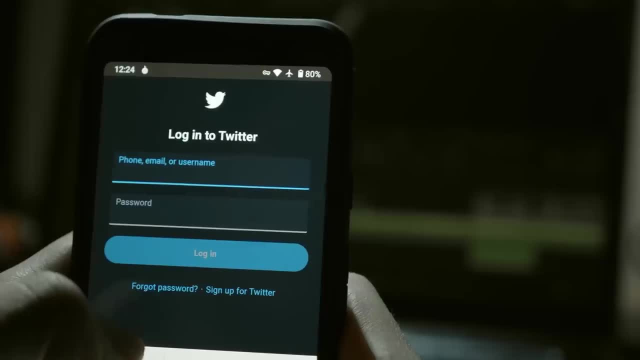 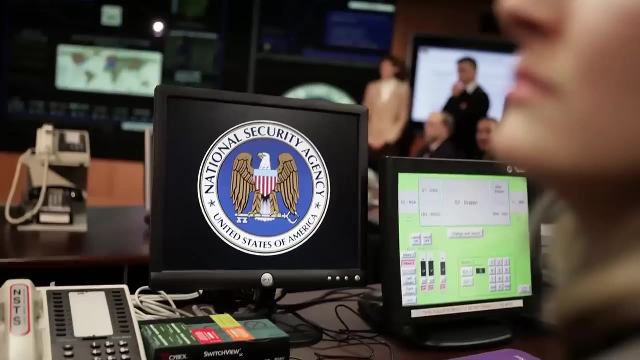 Do not log in to any online accounts through Tor unless they were created completely anonymously, And remember that Tor is essential, but it's not all. you need to be anonymous online. You can still be targeted by powerful adversaries. The main point of using Tor is to enjoy the 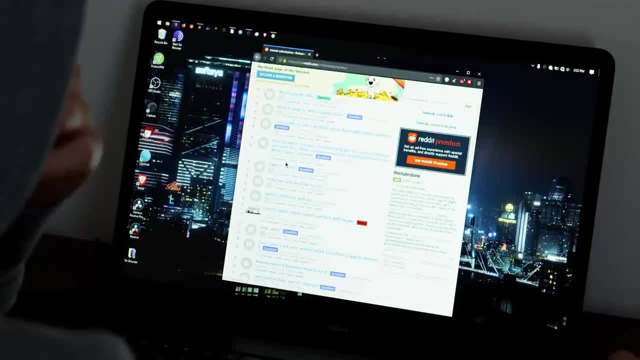 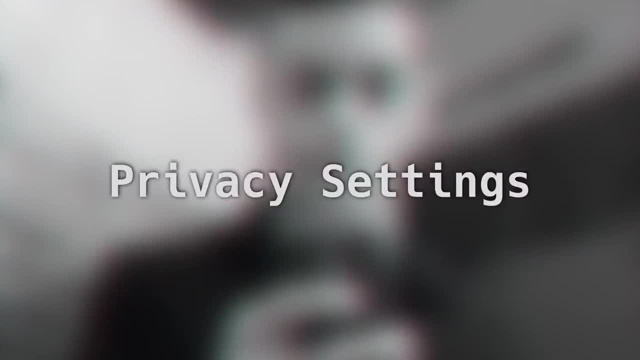 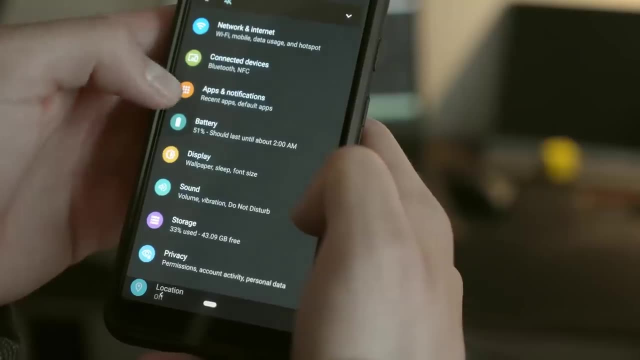 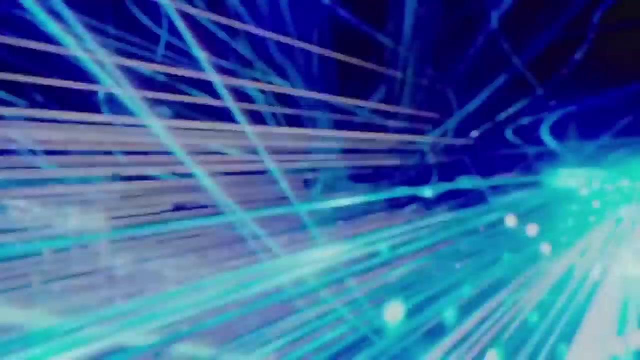 feature. Step number six: revise privacy settings. The next step involves a little bit more nuance than just simple tab to install. You need to go through the privacy settings of every app and account you sign up for and opt out of any data sharing or marketing consent. 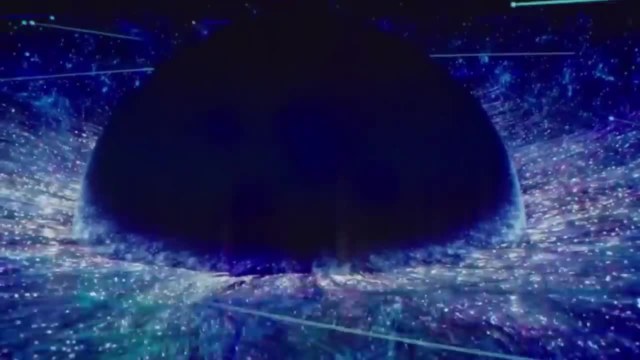 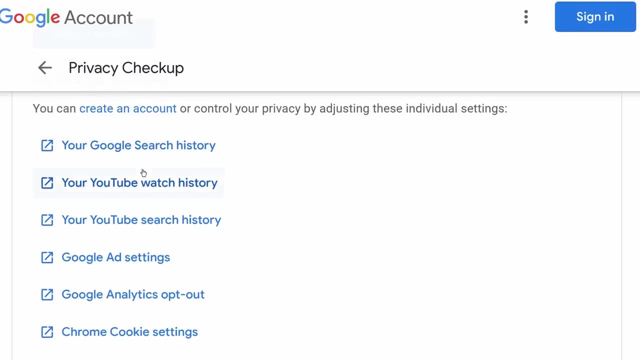 You'd be surprised how much you're exposed simply by having these settings toggled in the wrong way. Most of this is unnecessary and opting out won't affect your user experience. Go through your Google account web and app activity settings. Apple ID privacy settings. 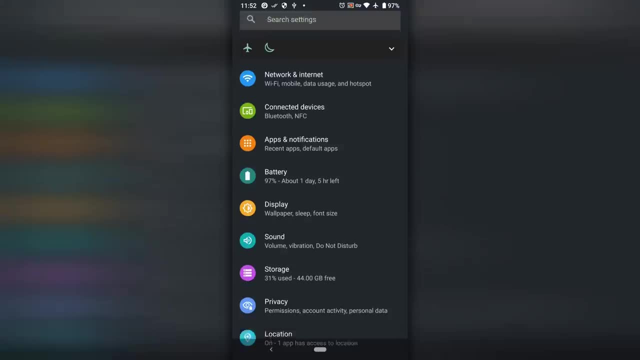 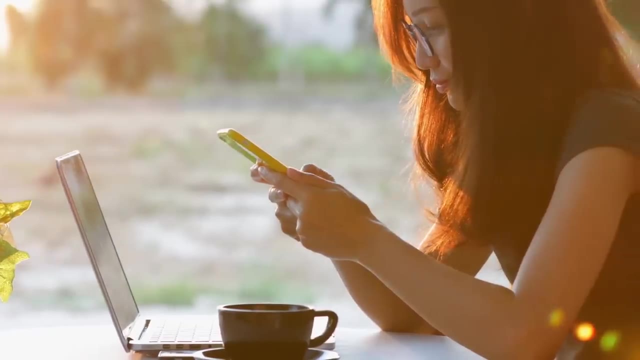 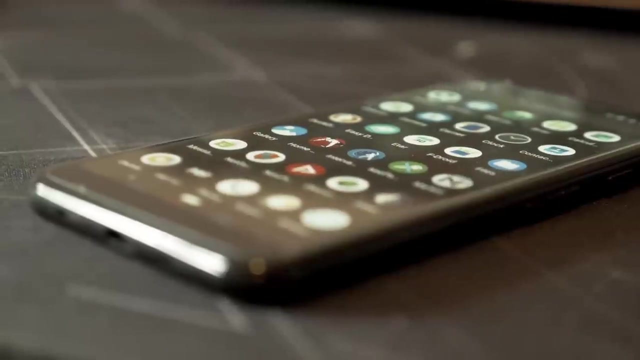 location services, Facebook, privacy and security, etc. Some of these settings may be hidden in the vague wording, such as personalization, allow suggestions and stuff like that. Make sure to do this on all your devices, apps and accounts. Step number seven: while you're revising your privacy settings, take a minimalist approach. 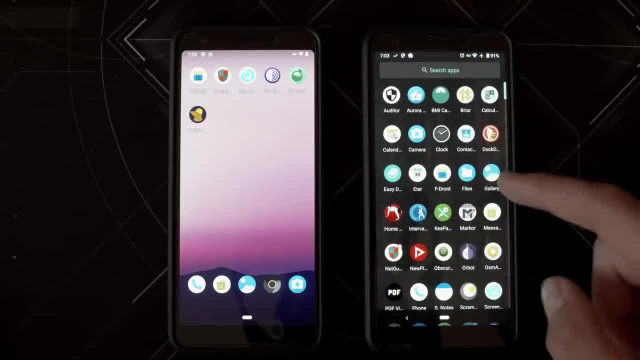 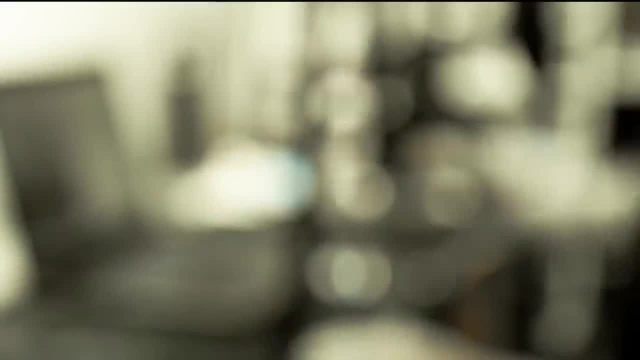 to your app setup. Chances are you have plenty of apps on your phone that are just sitting there collecting your data Without even opening the app for weeks. The more apps you install, the more exposed you are to data leaks and security risks.